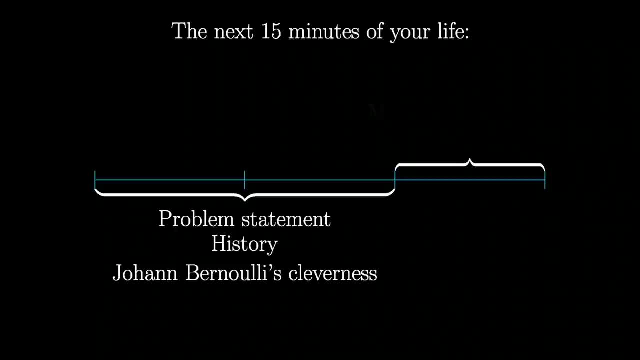 I'm going to show this proof that Steve showed me. It's by a modern mathematician, Mark Levy, and it gives a certain geometric insight to Johann Bernoulli's original solution. And at the very end I have a little challenge for you. 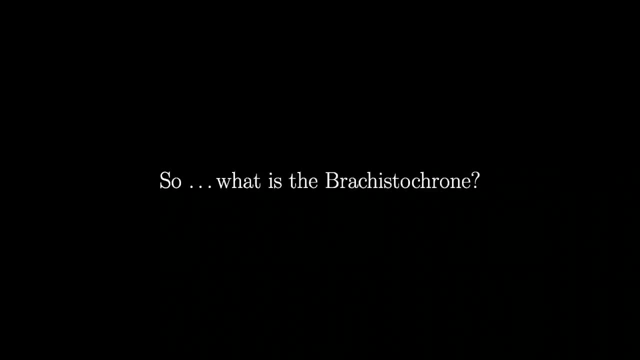 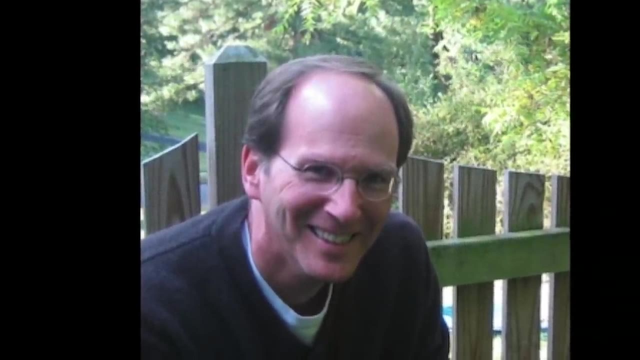 We should probably start off by just defining the problem itself. Okay, All right, You want me to take a crack at that? Yeah, go for it. Okay, Yeah. So it's this complicated word, first of all, Brachistochrone, that comes from two. 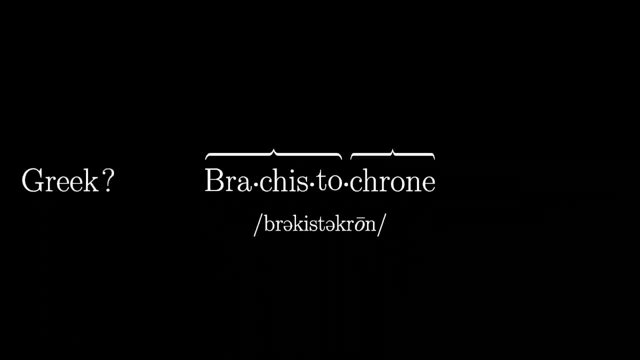 Gee, I have to check. Are those Latin or Greek words? I think I'm pretty sure they're Greek. Okay, So Greek words for the shortest time. and it refers to A question that was posed by one of the Bernoulli brothers, by Johann Bernoulli. 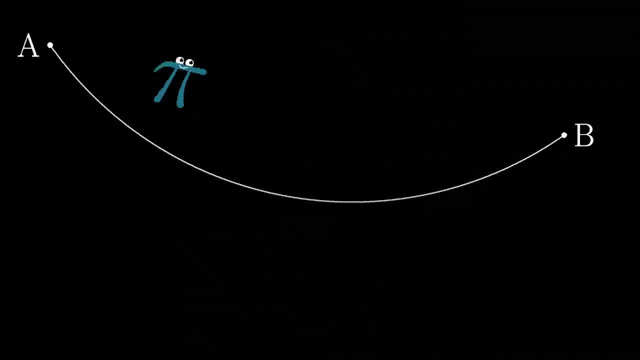 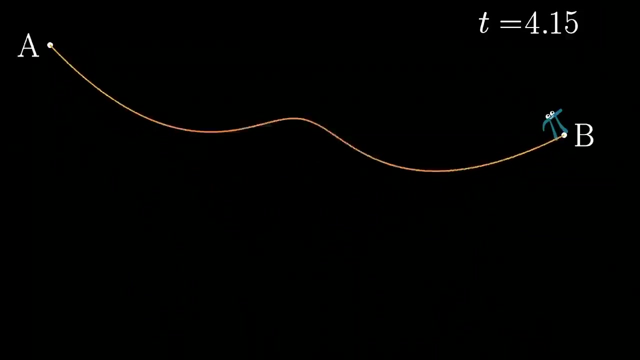 If you imagine like a chute, and there's a particle moving down a chute, being pulled by gravity, what's the path of the chute that connects two points so that it goes from point A to point B in the shortest amount of time. I think what I like most about this problem is that it's relatively easy to describe. 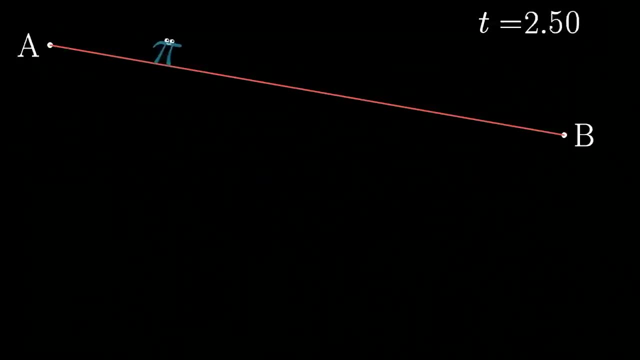 qualitatively what you're going for. You know you want the path to be short, something like a straight line, Mm-hmm, But you want the object to get going fast, which requires starting steeply and that adds length to your line. 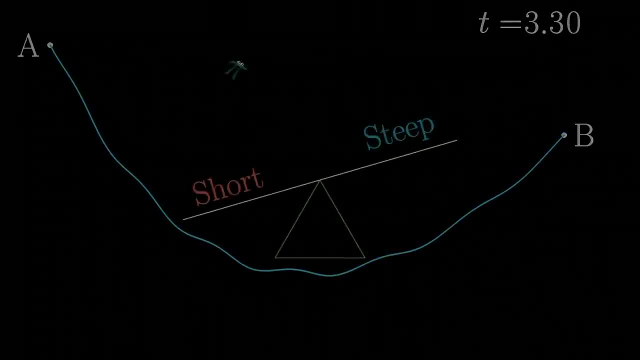 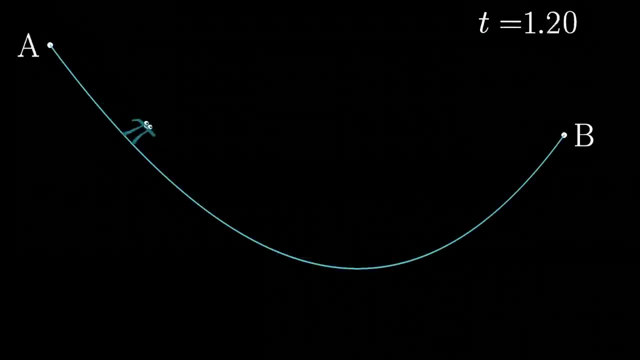 Mm-hmm. But making this quantitative and actually finding the balance with a specific curve, it's not at all obvious and makes for a really interesting problem. It is. It's a really interesting thing- I mean most people- when they first hear it. 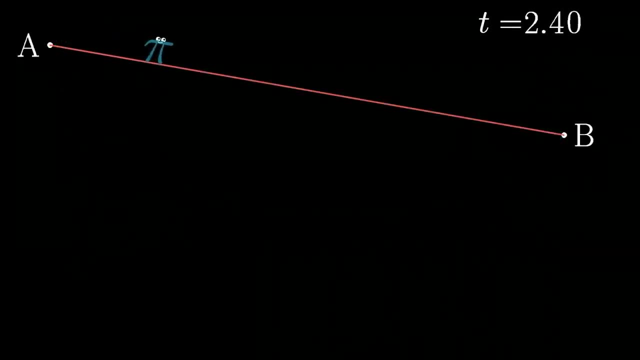 assume that the shortest path will give the shortest time, that the straight line is the best. But, as you say, it can help to build up some steam by rolling straight down at first- or not necessarily rolling, I mean it. You could picture it sliding, That doesn't really matter how we phrase it. But 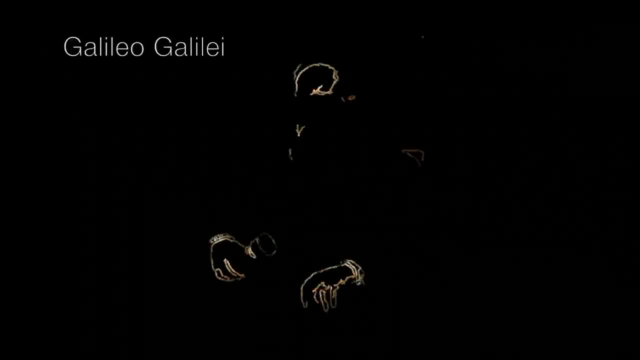 So Galileo had thought about this himself much earlier than Johann Bernoulli in 1638.. And Galileo thought that an arc of a circle would be the best thing. So he had the idea that a bit of curvature might help. And it turns out that the arc of the circle is not the right answer. 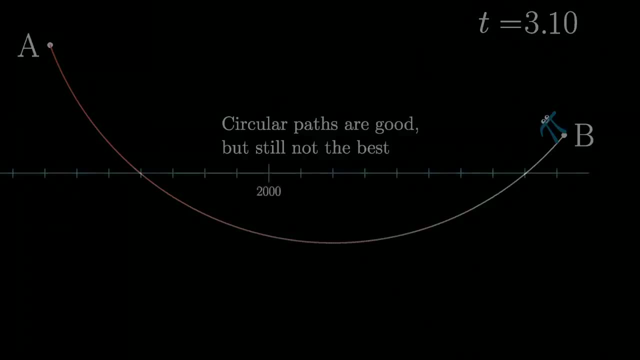 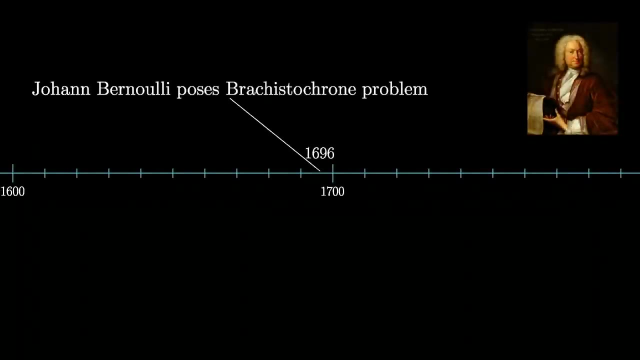 It's good, but there are better solutions And the history of real solutions starts with Johann Bernoulli posing this as a challenge. So that's then in In June of 1696.. And he posed it as a challenge really to the mathematical world at that time. 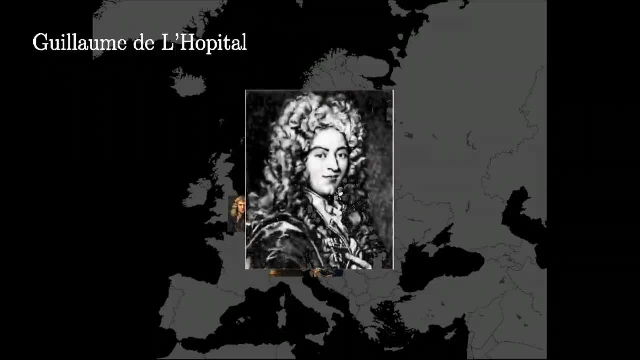 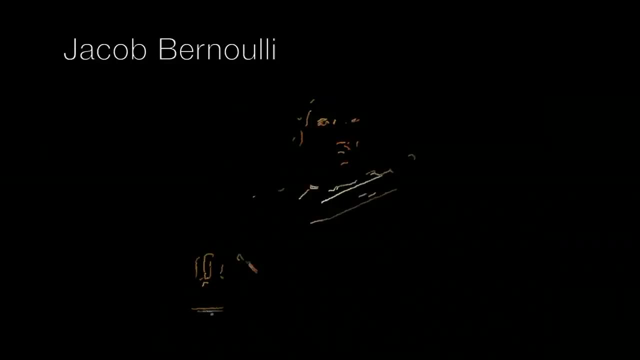 For him that meant the mathematicians of Europe, And in particular, he was very concerned to show off that he was smarter than his brother, you know. So he had a brother, Jacob, and the two of them were quite bitter rivals actually. 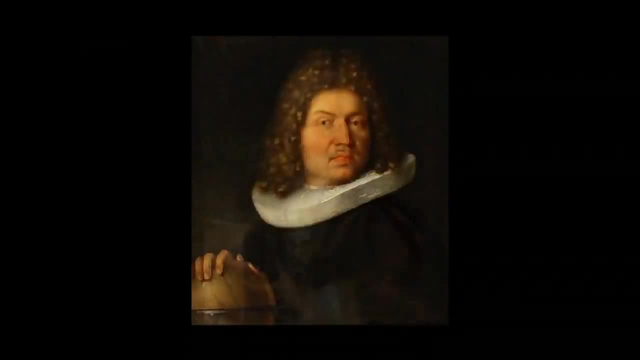 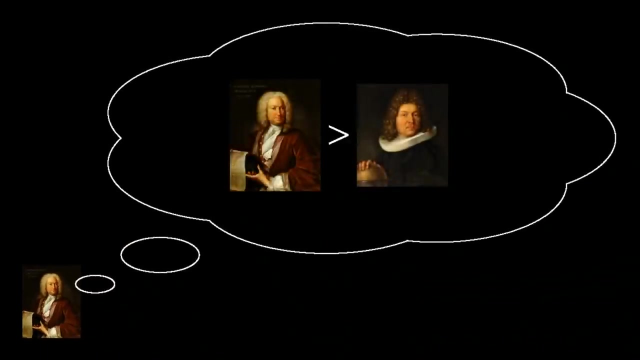 both tremendous mathematicians. But Johann Bernoulli fancied himself the greatest mathematician of his era, not just better than his brother, but, You know, I think he thought that he might be better than Leibniz, who was alive at the time. 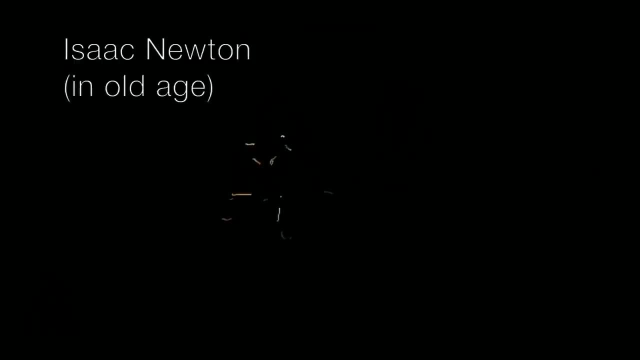 and Isaac Newton, who was by then sort of an old man, I mean more or less retired from doing math. Newton was the Warden of the Mint, Be something like Secretary of the Treasury nowadays. And Newton shows him up right. 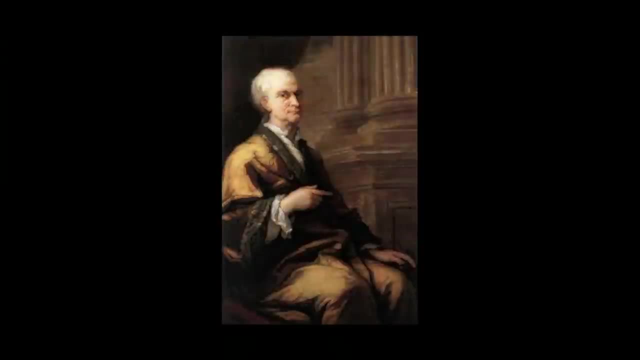 He stays up all night and solves it, even though it took Johann Bernoulli two weeks to solve. That's right. That's the great story that Newton was shown the problem. It wasn't really. He wasn't really pleased to be challenged, especially by somebody that he considered. 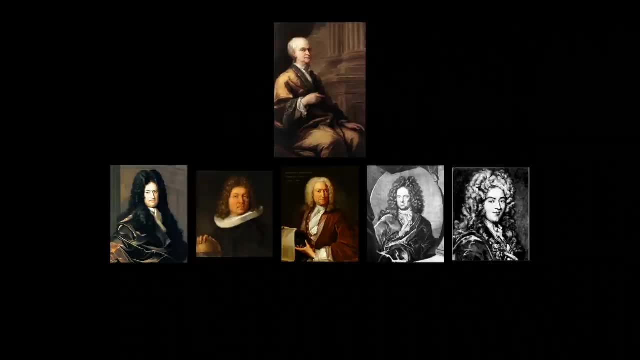 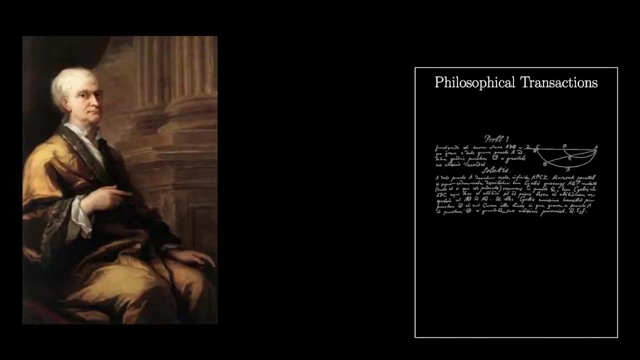 beneath him. I mean he considered pretty much everybody beneath him. But yeah, Newton stayed up all night, solved it and then sent it in anonymously to the Philosophical Transactions, the journal at the time, And it was published anonymously. And so Newton complained in a letter to a friend of his. 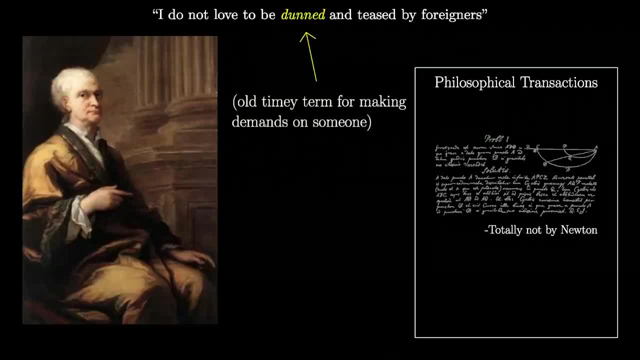 He said: I do not love to be dunned and teased by foreigners about mathematical things. So he didn't enjoy this challenge, but he did solve it. The famous legend is that Johann Bernoulli, on seeing this anonymous solution, said: 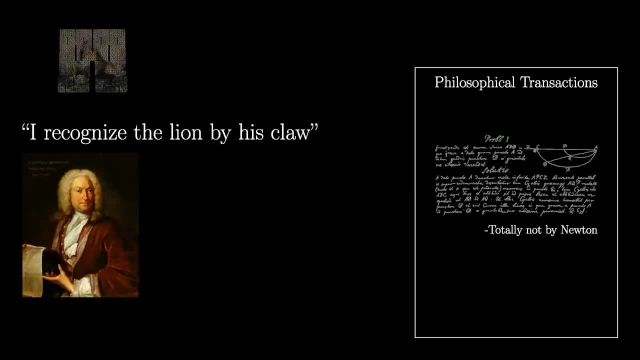 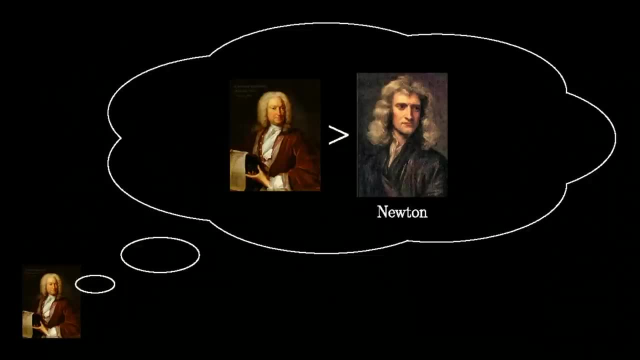 I recognize the lion by his claw. I don't know if that's true, but it's a great story. Everyone loves to tell that story And I suspect part of the reason that Johann was so eager to challenge other mathematicians like Newton is he secretly knew that his own solution was unusually clever. 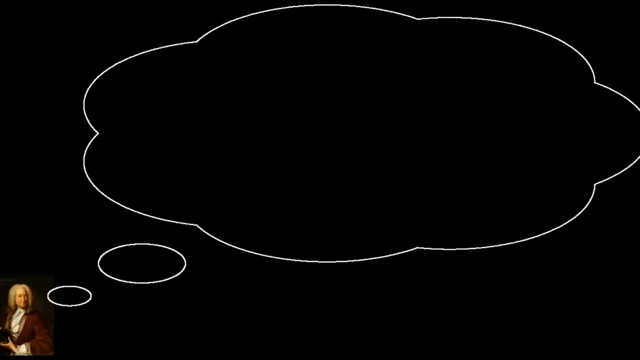 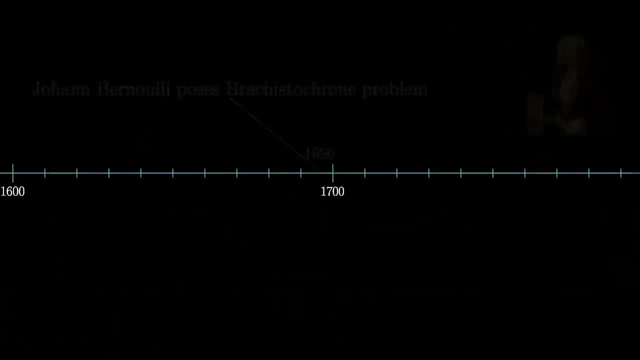 Maybe we should start going into what he does, Mm-hmm, Yes, Yeah, He imagines that to solve the problem, you let light take care of it for you, Because Fermat in the early 1600s had shown that you could state the way that light travels. 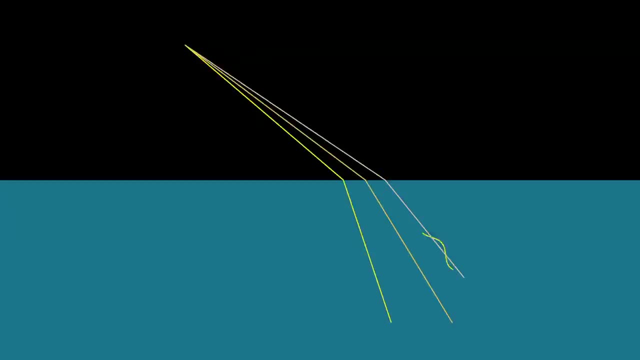 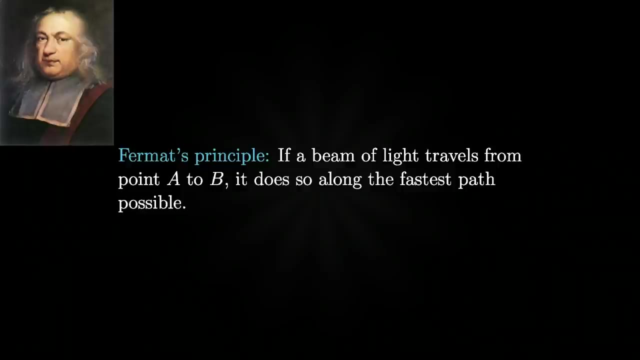 whether bouncing off of a mirror, or refracting from air into water where it bends, or going through a lens, all the motion of light could be understood by saying that light takes whatever path, gets it from point A to point B in the shortest time, Which is a really awesome perspective when you think about it. 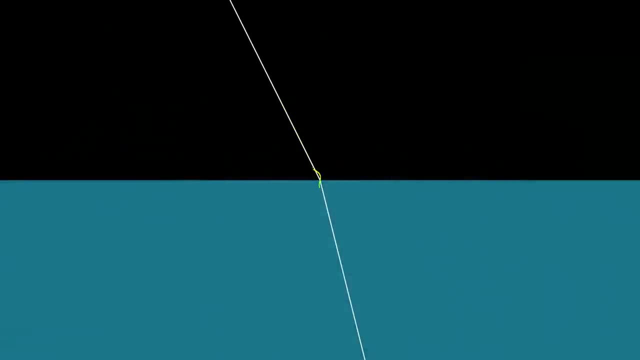 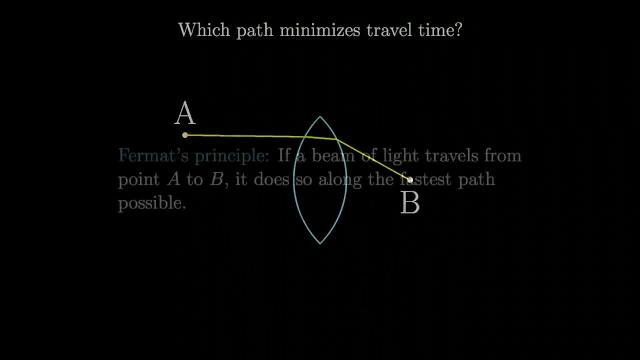 Because usually you think very locally in terms of what happens to a particle at each specific point. This steps back and looks at all possible paths and says: nature chooses the best one. Yes, it is. It's a beautiful and, as you say, really an awe-inspiring mental shift for some people. 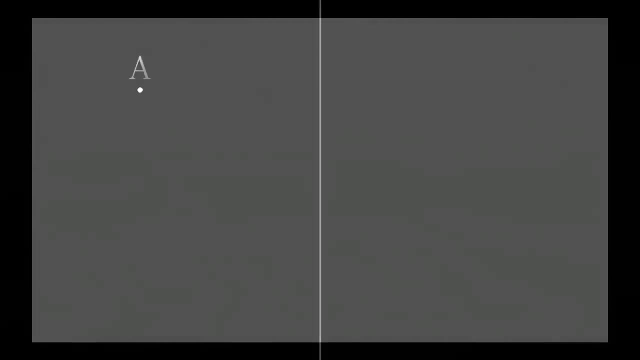 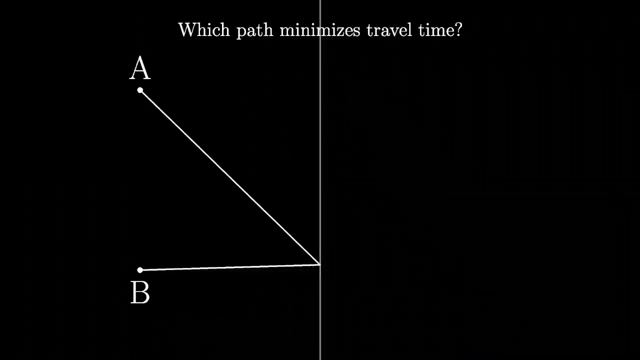 Literally awe-inspiring, in the sense that it had religious overtones, that somehow nature is imbued with this property of doing the most efficient thing. Oh, interesting. But leaving that aside, you know, you've seen it, you know, you could just say: it's an empirical fact that that is how light behaves, And so 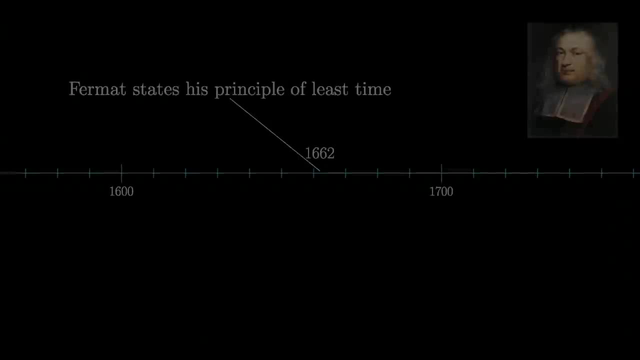 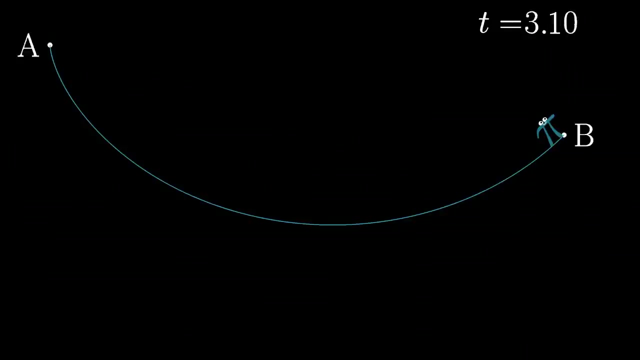 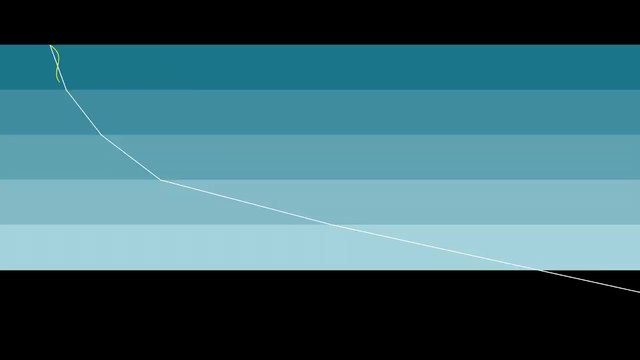 Johann Bernoulli's idea was to then use Fermat's principle of least time and say: let's pretend that instead of a particle sliding down a chute, it's light traveling through media of different index of refraction, meaning that the light would go at different speeds as it successively went. 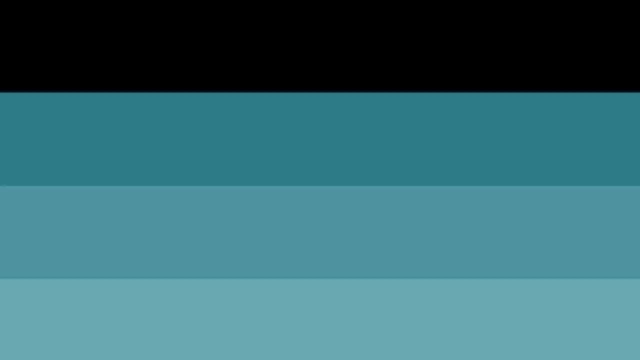 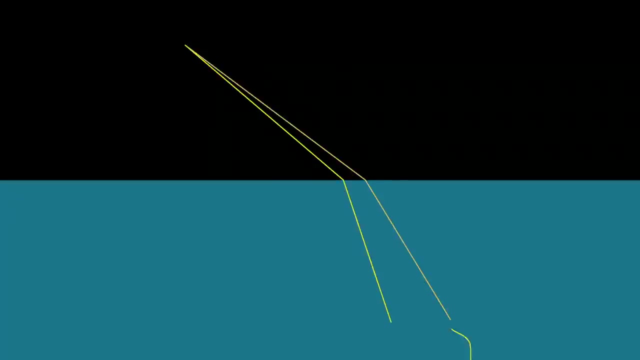 sort of down the chute, And I think before we dive into that case we should look at something simpler. So at this point in the conversation we talked for a while about Snell's law. This is a result in physics that describes how light bends when it goes from one material into. 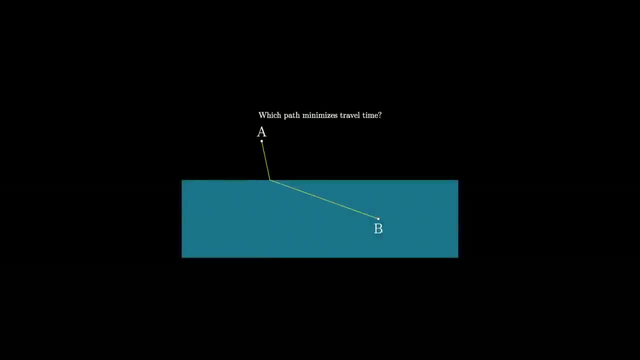 another, where its speed changes. I made a separate video out of this, talking about how you can prove it using Fermat's principle, together with a very neat argument using imaginary constant tension springs, But for now, all you need to know is the statement of Snell's law itself. 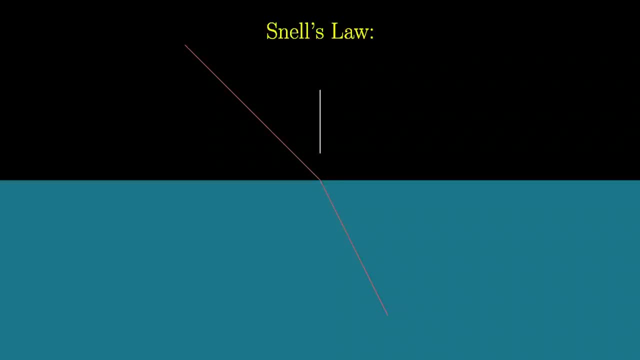 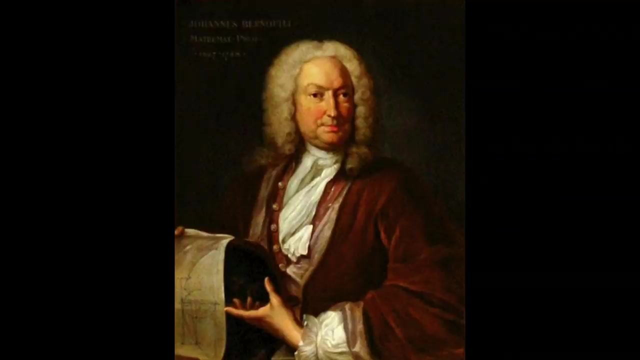 When a beam of light passes from one medium into another and you consider the angle that it makes with a line perpendicular to the boundary between those two materials, the sine of that angle, divided by the speed of light, stays constant as you move from one medium to the next. So what? 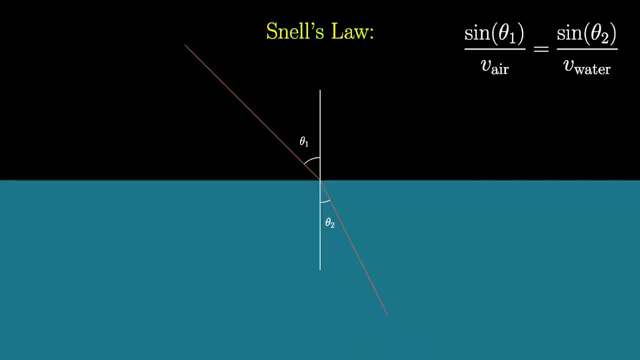 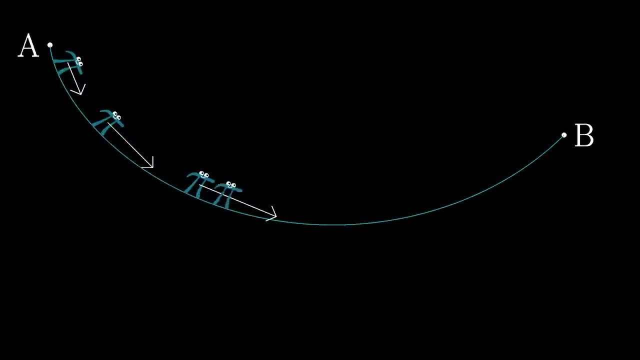 Johann Bernoulli does is find a neat way to take advantage of that fact. this sine of theta over v stays constant, fact for the Brachistochrone problem, And when he thinks about what's happening with the particle sliding down the chute. 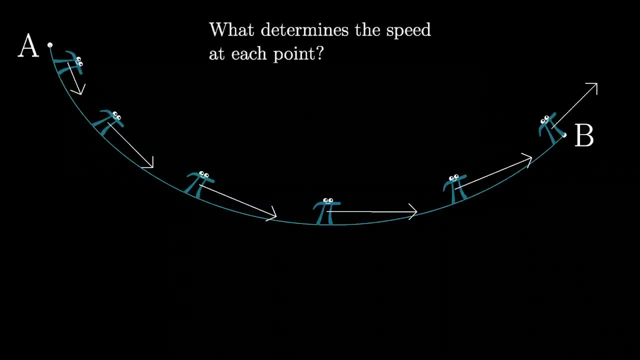 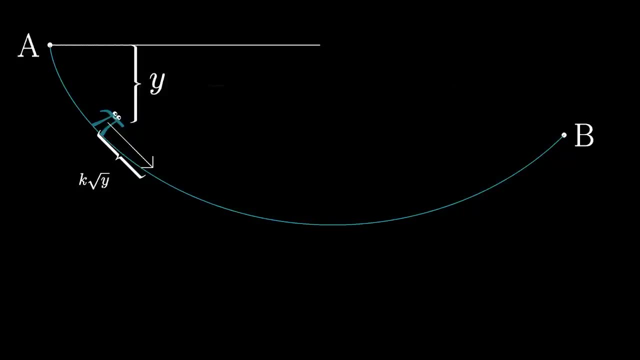 he notices that by conservation of energy, the velocity that the particle has will be proportional to the square root of the distance from the top. And just to spell that out a little bit more, the loss in potential energy is its mass times, the gravitational constant times, y, that distance from the top. And when you set that equal to the 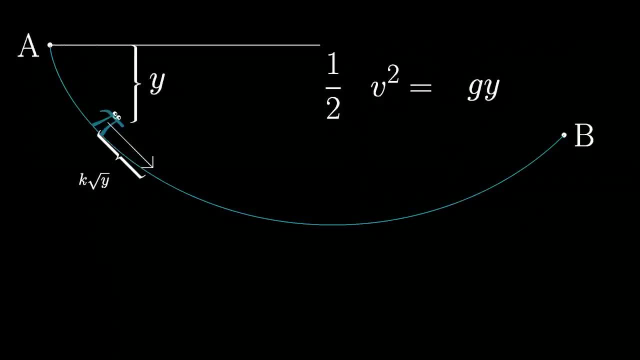 kinetic energy one half times mv squared, and you rearrange, the velocity, v will indeed end up being proportional to the square root of y. Yes, So that then gives him the idea about- let's imagine- glass of many different layers, each with a different velocity characteristic for the light in it. 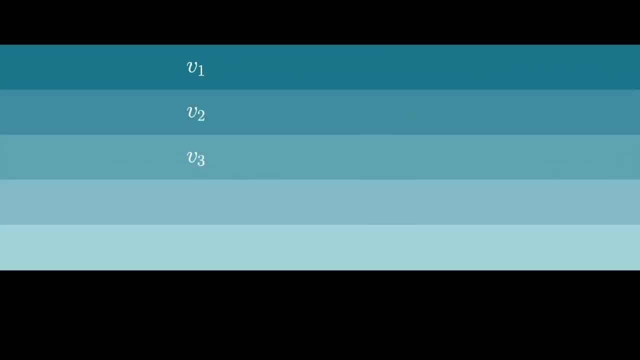 The velocity in the first one is v1, and the next one is v2, and the next one is v3, and these are all going to be proportional to the square root of y1 or y2 or y3.. And in principle, you should be thinking about a limiting process where you have 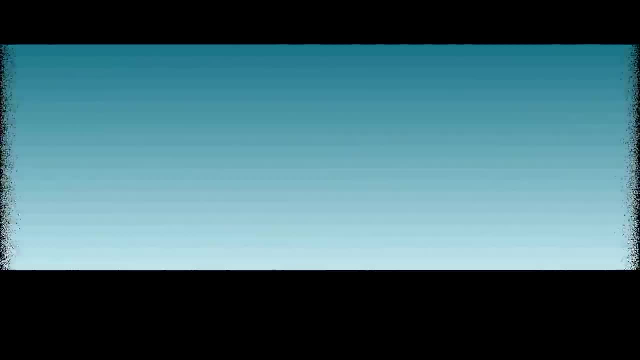 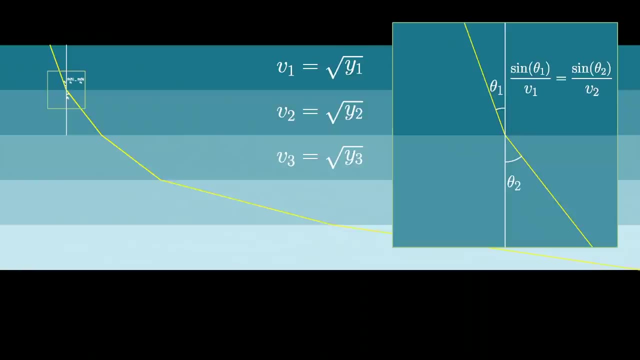 infinitely many, infinitely thin layers, and this is kind of a continuous change for the speed of light. And so then his question is if light is always instantaneously obeying Snell's law as it goes from one medium to the next, so that v over sine theta is always a constant as I move. 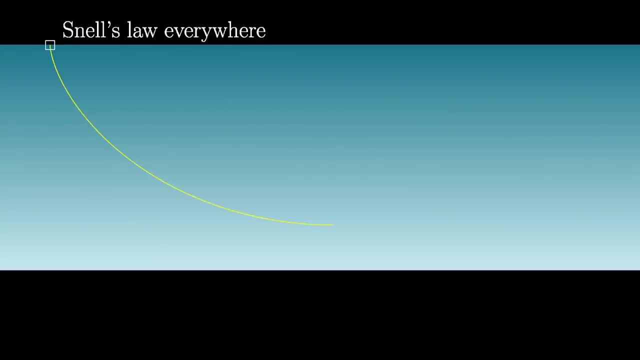 from one layer to the next. what is that path where you know, such that these tangent lines are always instantaneously obeying Snell's law? And for the record, we should probably just state exactly what that property is? Okay, So the conclusion that Johann made was that, if you look at, whatever the time-minimizing curve is, 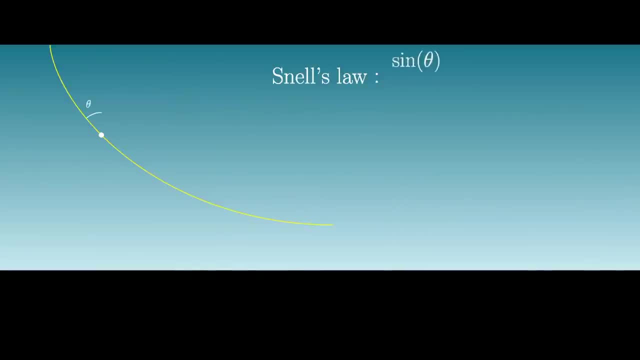 and you take any point on that curve, the sine of the angle between the tangent line at that point and the vertical divided by the square root of the vertical distance between that point and the start of the curve. that's what you get, Okay. 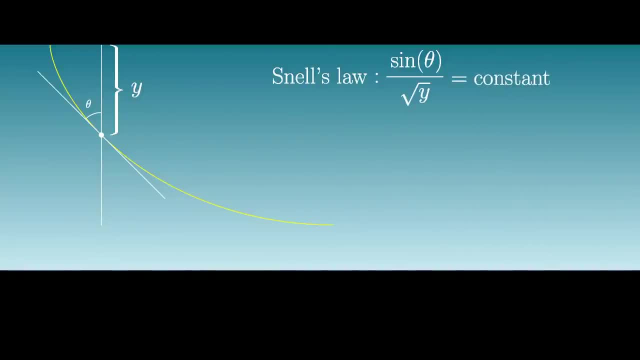 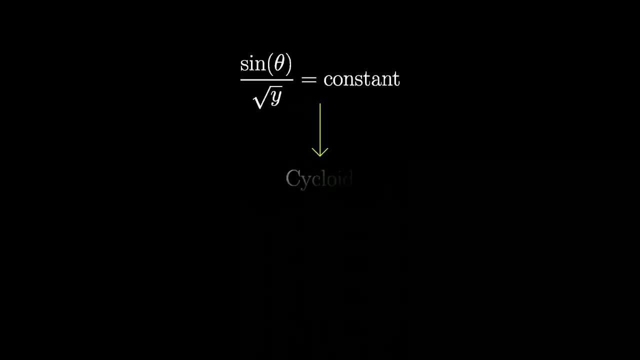 Okay, So that's going to be some constant, independent of the point that you chose. And when Johann Bernoulli first saw this- correct me if I'm wrong- he just recognized it as the differential equation for a cycloid, the shape traced by the point on the rim of a rolling wheel. 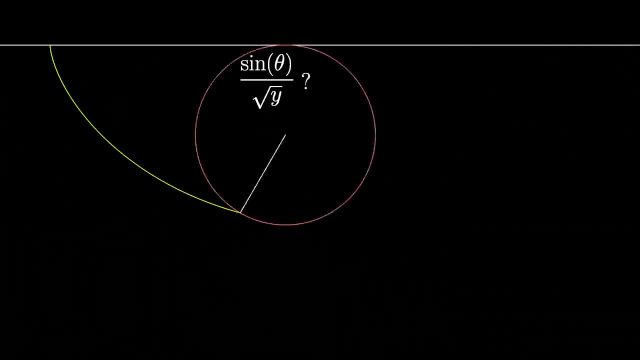 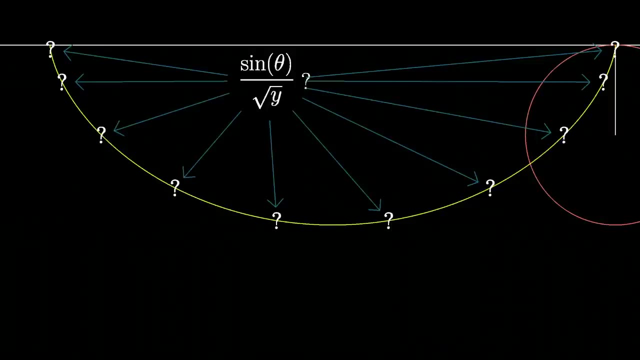 But it's not obvious- certainly not obvious to me- why this sine of theta over square root y property has anything to do with rolling wheels. It's not at all obvious. but this is again the genius of Mark Levy to the rescue. 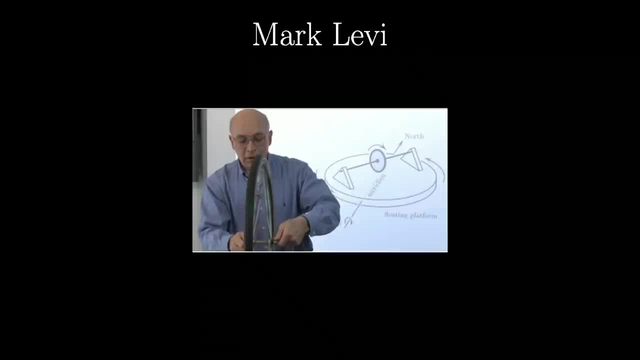 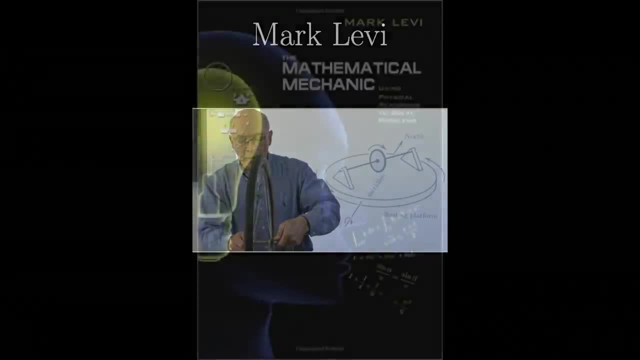 You want to say a few words about Mark Levy. Yeah Well, Mark Levy is a very clever as well as a very nice guy who's a friend of mine and a terrific mathematician at Penn State who has written a book called The Mathematical Mechanic. 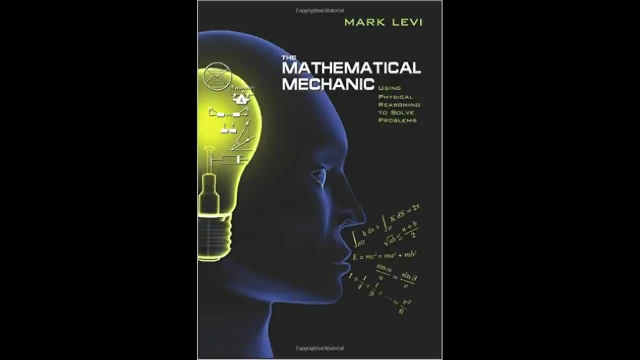 in which he uses principles of mechanics and, more generally, physics, to solve all kinds of math problems. That is rather than math in the service of science. it's science in the service of math. And as an example of the kinds of clever things that he's, 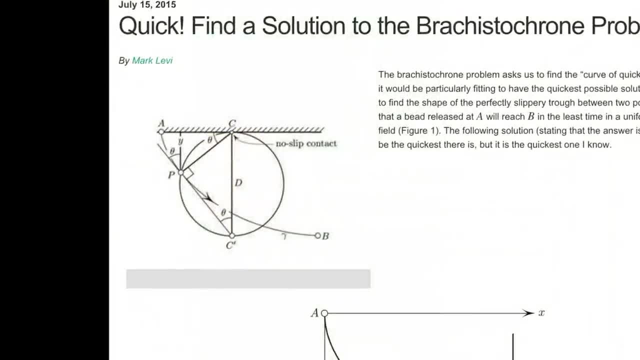 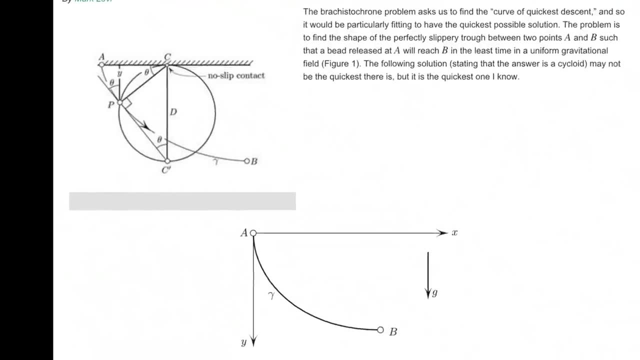 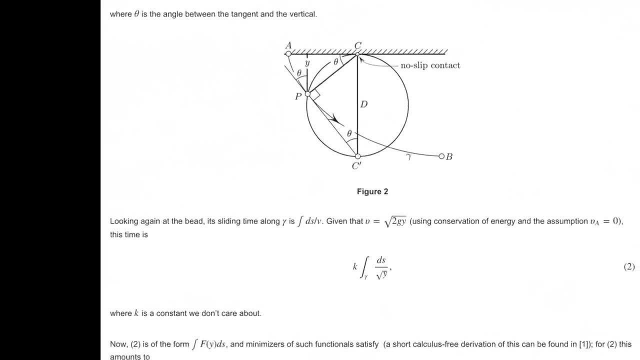 done and the kinds of things that he does. he recently published a little note, very short, showing that if you look at the geometry of a cycloid, just drawing the correct lines in the right places, that this principle of velocity over sine theta being constant is built in to. 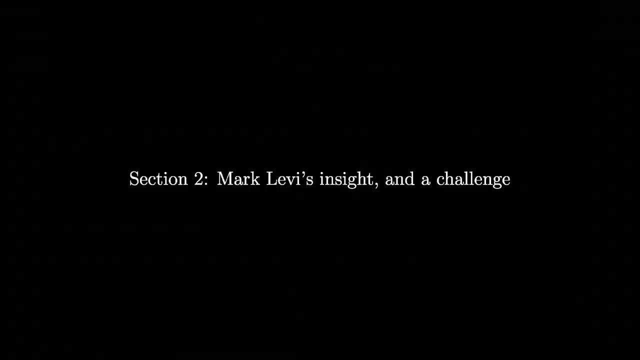 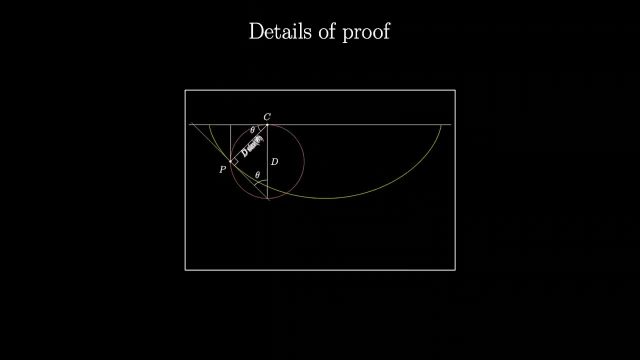 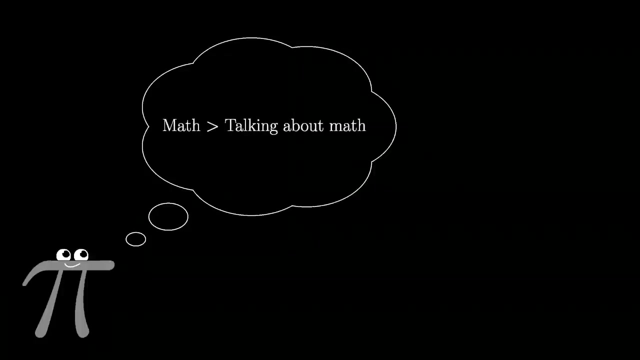 the motion of the cycloid itself. So in that conversation we never actually talked about the details of the proof itself. It's kind of a hard thing to do without visuals, But I think a lot of you out there enjoy seeing the math and not just talking about the math. It's also a really elegant little piece of geometry. 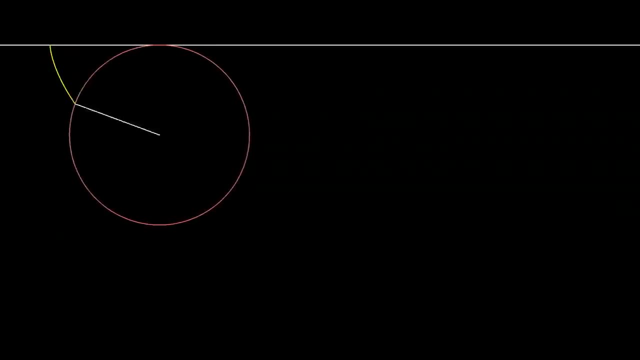 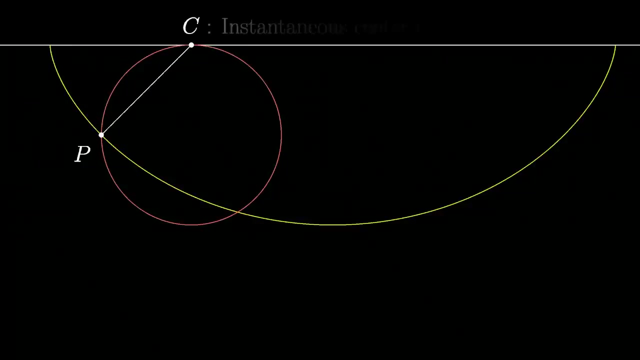 So I'm going to go through it here. Imagine a wheel rolling on the ceiling and picture a point P on the rim of that wheel. Mark Levy's first insight was that the point where the wheel touches the ceiling, that I'll call C, acts as this instantaneous center of rotation for the 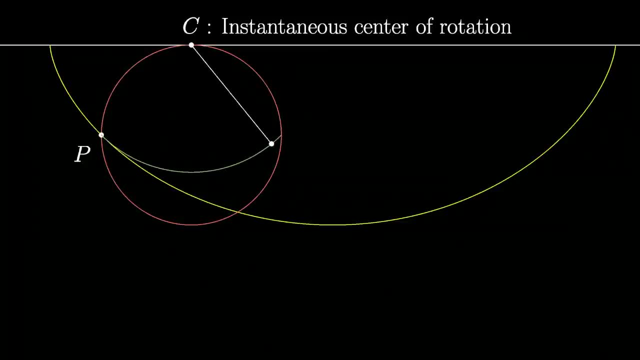 trajectory of P. It's as if, for that moment, P is on the end of a pendulum whose base is at C. Since the tangent line of any circle is always perpendicular to the radius, the tangent line of the cycloid path of P is perpendicular to the line PC. 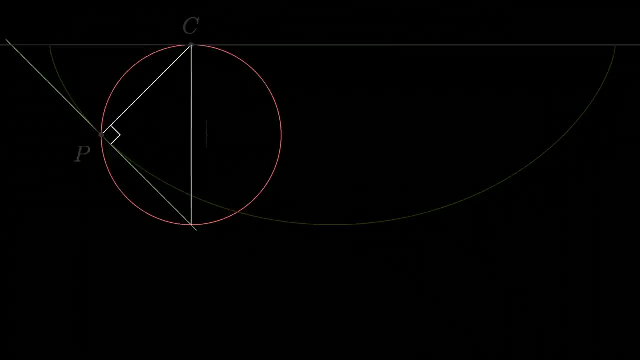 This gives us a right angle inside of the circle, and any right triangle inscribed in a circle must have the diameter as its hypotenuse. So from that you can conclude that the tangent line always intersects the bottom of the circle. Now let theta be the angle between this tangent line. 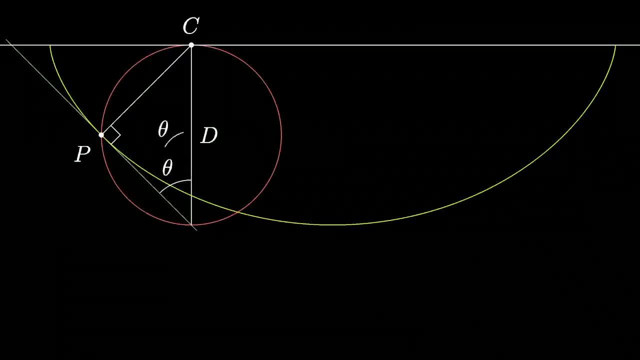 and the vertical. We get a pair of similar triangles which I'll just show on the screen. You can see that the length of PC is the diameter times sine of theta. Using the second similar triangle, this length times sine of theta again gives the distance between P and the. 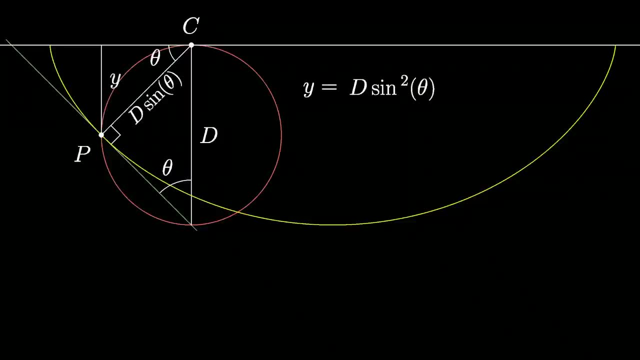 ceiling the distance that we were calling y earlier. Rearranging this, we see that sine of theta divided by the square root of y is equal to 1 divided by the square root of the diameter, Since the diameter of a circle, of course, stays constant throughout the rotation. 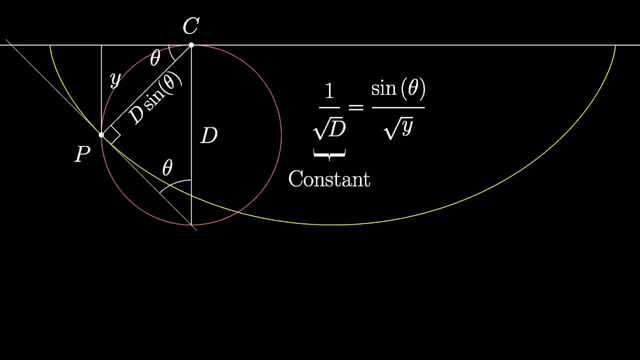 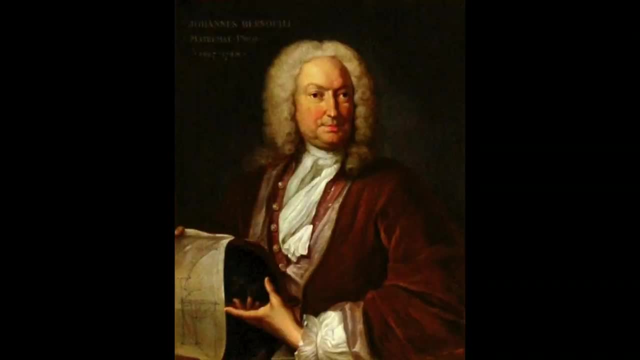 this implies that the sine of theta, divided by square root of y, is constant on a cycloid, and that's exactly the Snell's Law property that we're looking for. So when you combine Johann Bernoulli's insight with this little geometry proof, that's the cleverest solution of the. 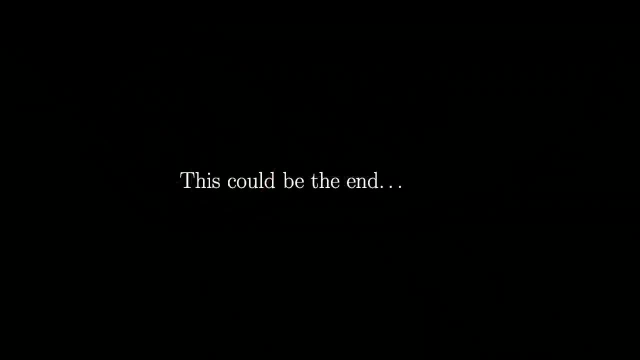 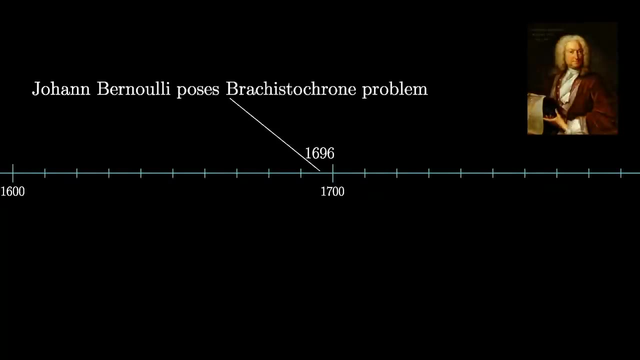 Brachistochrome that I've ever seen And I could call it done here. but given that the whole history of this problem started with a challenge that Johann Bernoulli posed, I want to finish things off with a little challenge of my own, When I was playing around with the equations. 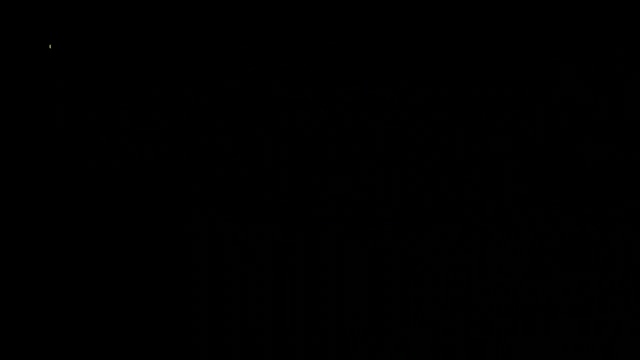 of a cycloid. something interesting popped out. Consider an object sliding down the cycloid due to gravity and think about where it is along the curve as a function of gravity. Now think about how the curve is defined as this trajectory of the point on the rim of a rotating 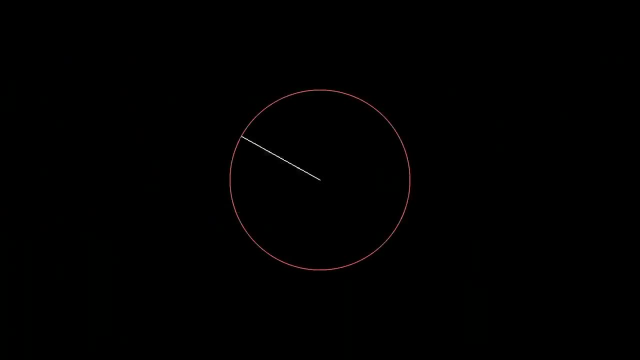 wheel. How might you tweak the rate at which the wheel rotates so that, when the object starts sliding, the marked point on the rim of the wheel always stays fixed to that sliding object? Do you start rotating it slowly and increase its speed? If so, according to what function? 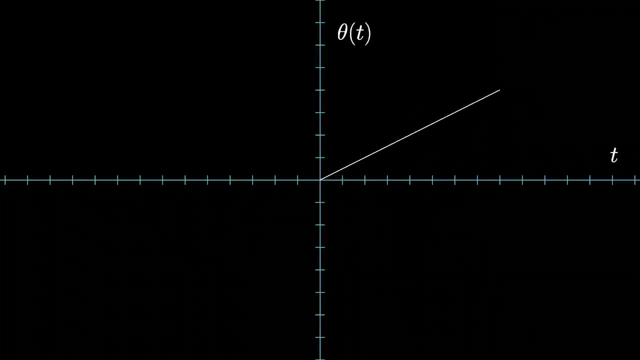 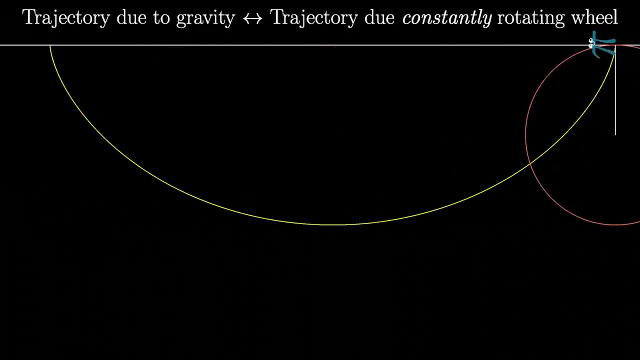 It turns out, it will rotate at a constant rate, which is surprising. This means that gravity pulls you along a cycloid in precisely the same way that a constantly rotating wheel would. The warm-up part of this challenge is just confirm this for yourself. 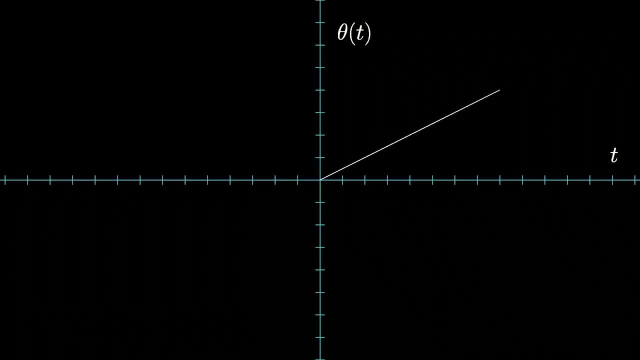 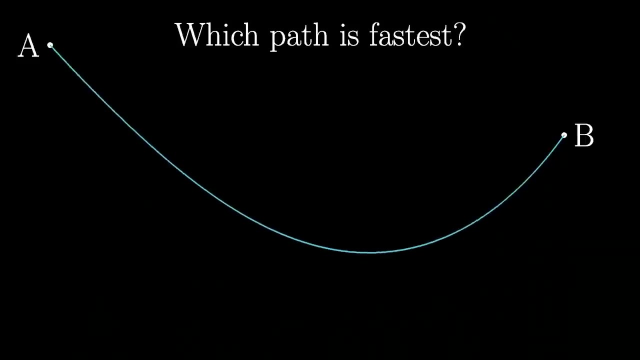 It's kind of fun to see how it falls out of the equations. But this got me thinking. If we look back at our original Brachistochrone problem, asking about the path of fastest descent between two given points, maybe there's a slick way to reframe our thinking. 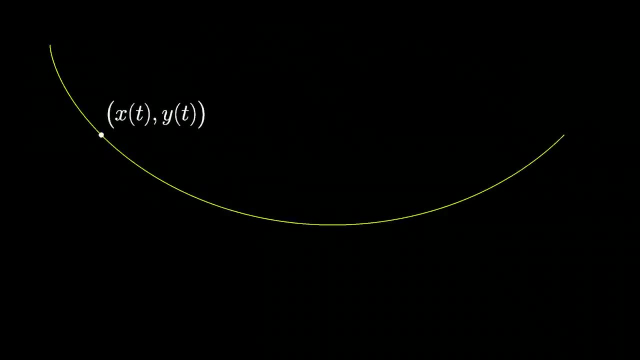 Instead of describing the trajectory of a sliding object in terms of its x and y coordinates, we described it in terms of the angle that the velocity vector makes as a function of time. I mean, you can imagine defining a curve by having an object start sliding. 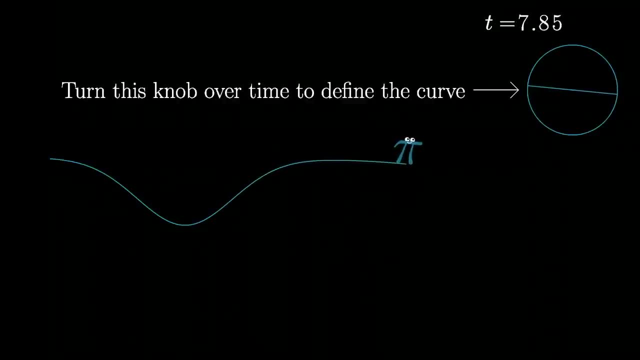 then turning a knob to determine the angle at which it's sliding at each point in time, always being pulled by gravity. If you describe the angle of the knob as a function of time, you are in fact uniquely describing a curve. You're basically using a. 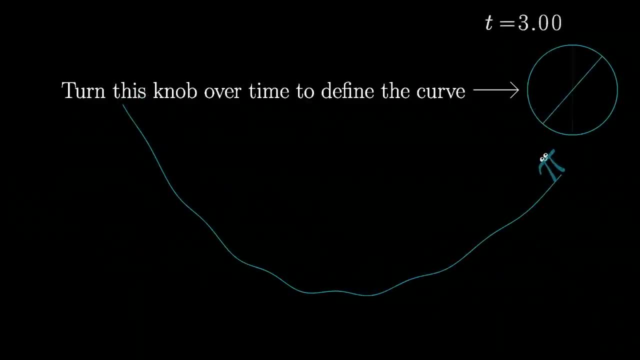 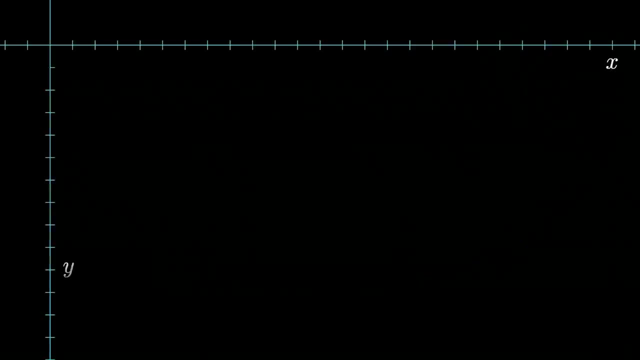 differential equation, since what's given is the slope as the function of some other parameter, in this case time. So what's interesting here is that when you look at the solution of the Brachistochrone problem not in the xy-plane, but in the t-theta plane, where t is time, 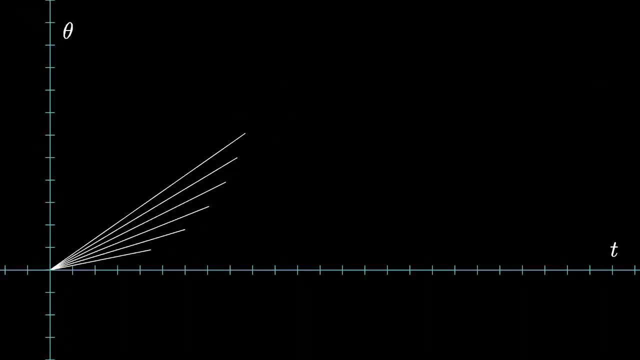 theta is the angle of the path. all of the Brachistochrone solutions are straight lines, That is to say, theta increases at a constant rate with respect to t When the solution of a curve minimization problem is a straight line. 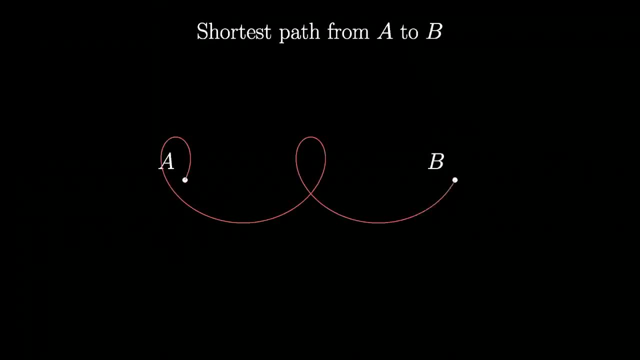 it's highly suggestive that there's some way to view it as a shortest path. problem. Here it's not so straightforward, since the boundary conditions that your object start at a point a and end at a point b in the xy-space doesn't just look like going from one point to. 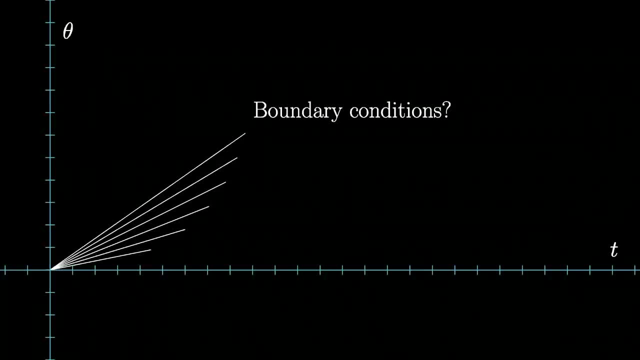 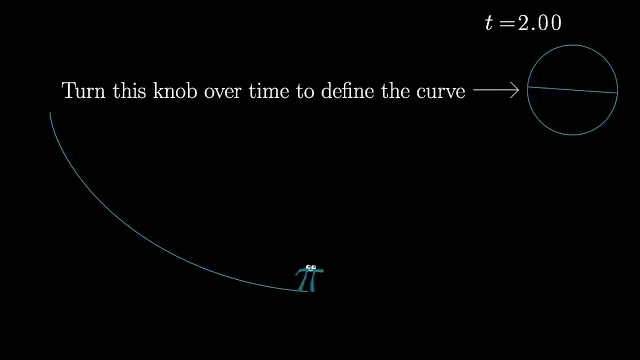 another in the theta t-space. Nevertheless, my challenge to you is this: Can you find another solution to the Brachistochrone problem by explaining why it must be the case that a time-minimizing trajectory, when represented in t-theta, is not a straight line but a point-to-point? data space looks like a straight line.